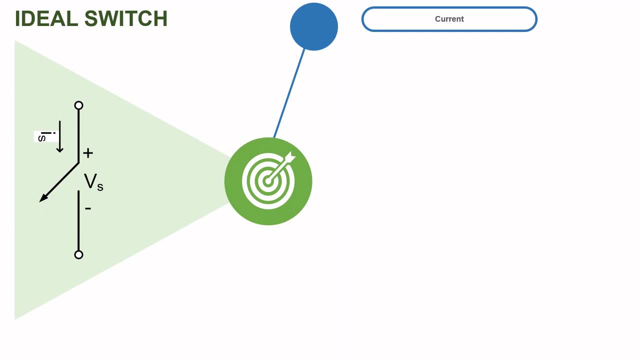 as well as reverse direction without causing any damage to the switch. An ideal switch should be capable of blocking infinite amount of voltage in forward and reverse direction, as well as reverse biased condition without causing any damage to the switch. Switching frequency: An ideal switch should be capable of operating at infinite timing. 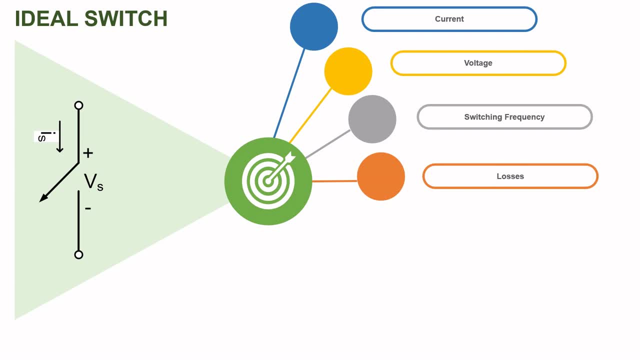 In case of the switch- other more fitting part- the ideal switching frequency should be able to be integrated into machine. Willy winner: from power information into power. thr McMillian o't table. it is in conduction mode or it is in dynamic mode that it is changing its state from on state to off? 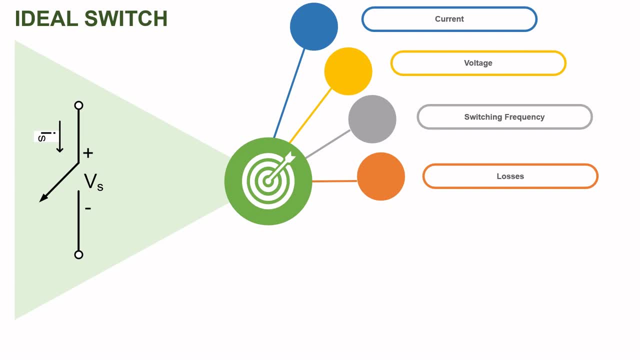 state or off state to on state. during all these periods, losses occurring inside the ideal switch should be equal to zero. the ideal switch should be 100 percent reliable. whenever the command is given to the switch, switch should operate and when the command is not given to the switch, 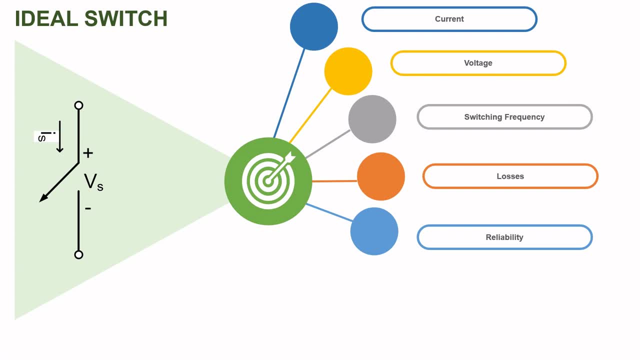 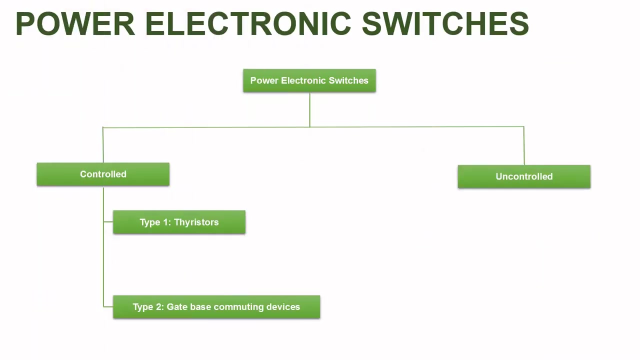 switch should not maloperate about size and construction. the size of the switch be as small as possible and the construction of the switch should be simple. If we are able to achieve all these properties in any of the switch, we can call that switch as an ideal switch. 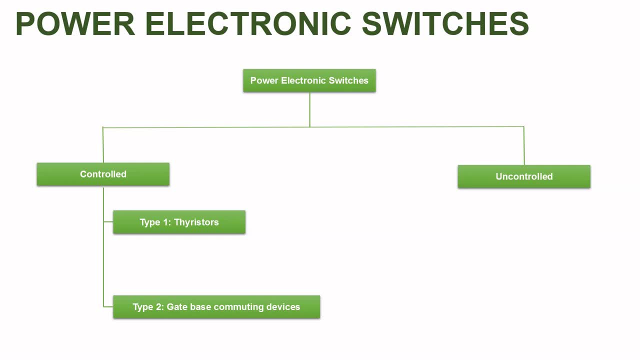 Power. electronic switches can be classified into two main categories: First is controlled switches and Second is uncontrolled switches. Control switches are those switches in which the turning on operation or turning off operation, or both the turning on and turning off operations, can be controlled by some electrical or electronic. 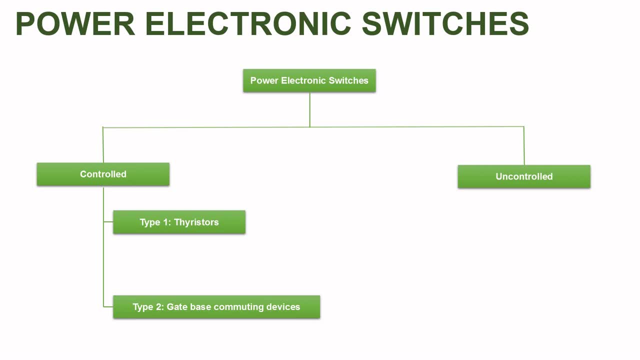 mechanisms ore. Both turning on and turning off operation cannot be controlled by any electrical or electronic mechanism. Controlled switches are further classified into two types. first type is thyristor. thyristors are the family of devices. In thyristor family devices mostly either turning on process is controlled or turning. 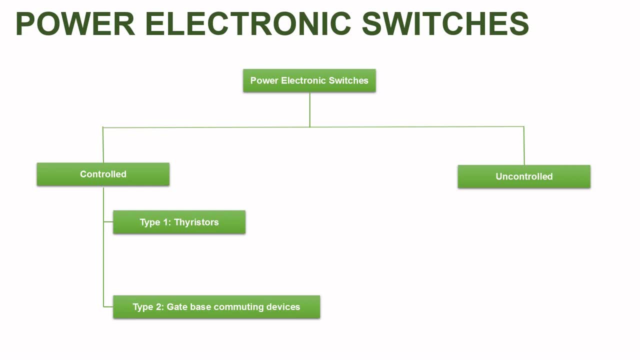 off process is controlled. both processes are not controlled in case of thyristor family devices. Thus these devices are usually called as semi-controlled devices, though some exceptions are existing in these devices also. 3. In type 2 devices we are having gate based commuting devices. 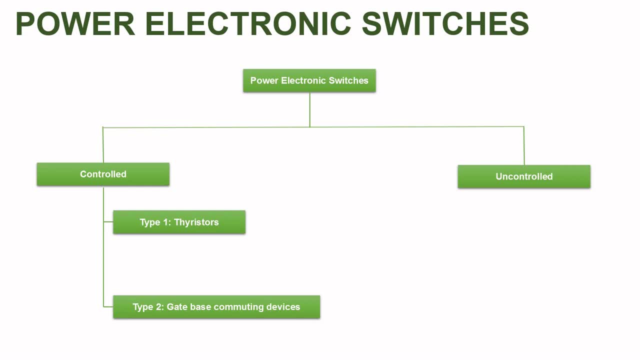 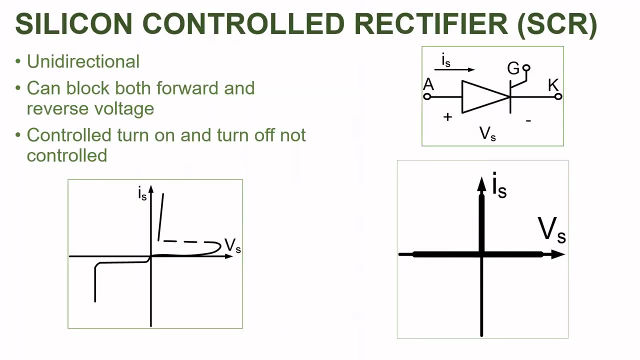 In these devices, both the turning on and turning off operation of the device is controlled. hence these devices are usually referred as fully controlled devices. 4. For first devices In type 2 devices: silicon controlled rectifier or SCR. SCR is a unidirectional device that 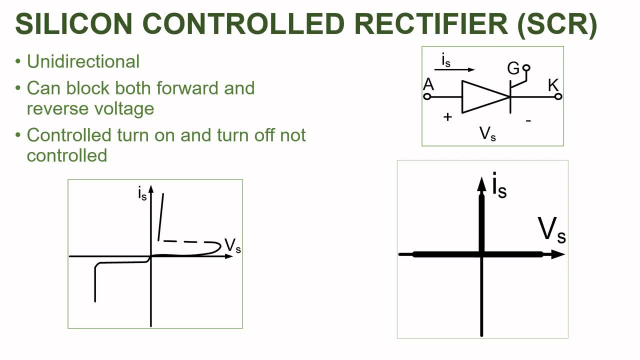 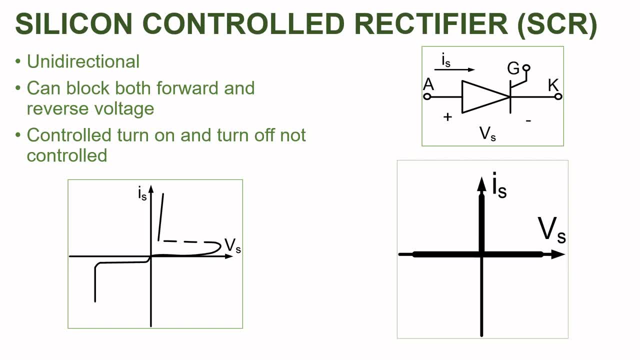 In type 2 devices And that's the 1- POW airthrough cell. during switching on and off, This DC current can generate voltage of its own circuit. with exactly specific towns of DC current, The turn-on process of SCR can be controlled if they are connected and in direct line to. 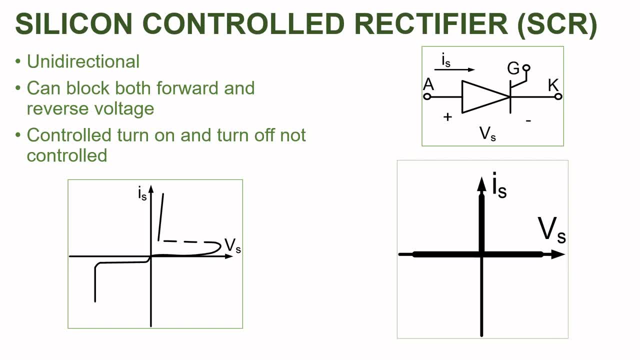 the gate they are connected to gate of its own C lines. Or if they are connected to wire, that cabinet jack would best be hasn't to the strange kind of level signals. Or if they are the transit of the signal, they should also have direct arc. 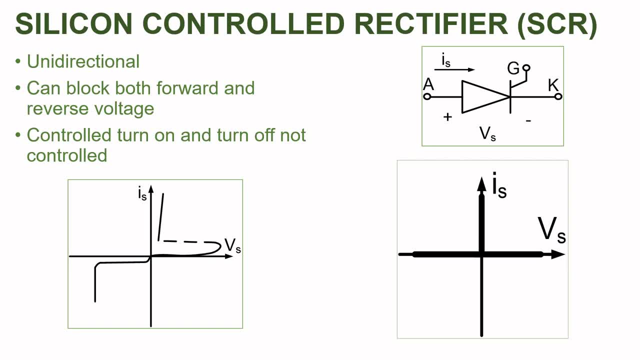 to the gate. Once the device is turned on, gate has got no control over the working of SCR. The characteristics of SCR are shown in this figure. Here we can see it is capable of blocking forward voltage as well as reverse voltage. but it can block forward as well as reverse voltage. 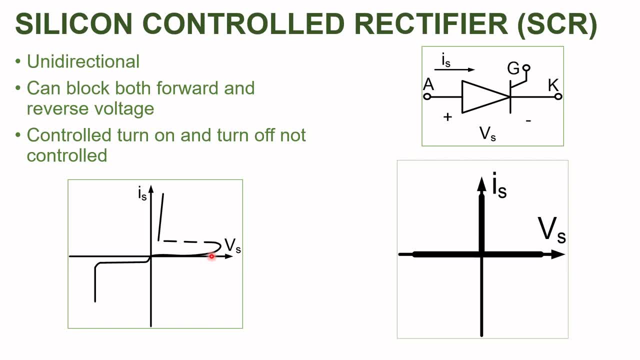 only up to a particular instant. This figure indicates the capabilities of SCR. Here we can see SCR can block forward voltage. SCR can also block reverse voltage. SCR can carry current in the forward direction, but SCR cannot carry current in the reverse direction. These values are limited. 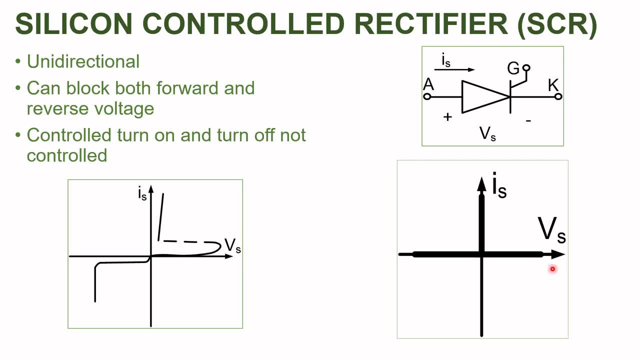 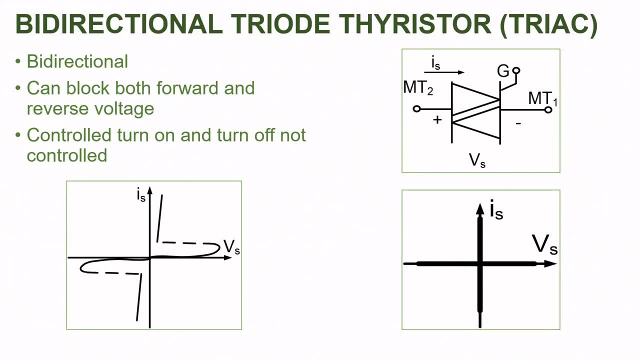 up to the rating of that particular SCR. So our next device is bidirectional triode thyristor, or TRIAC As the name indicates. it's a bidirectional device. that means current can flow from terminal MT2 to MT1 or from MT1 to MT2.. 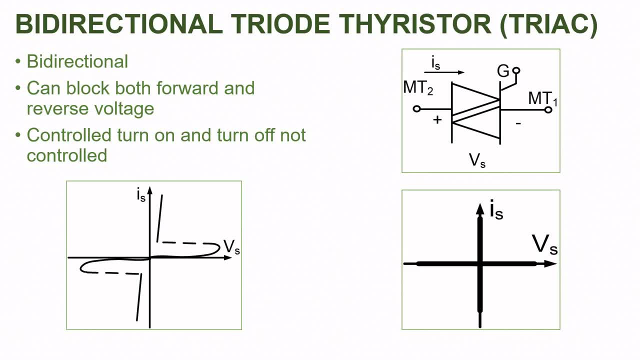 This device can block the voltages in both forward as well as reverse direction, but we usually do not call voltages as forward bias or reverse bias in case of TRIAC, since it's a bidirectional device. Hence we usually say voltages can be blocked when. 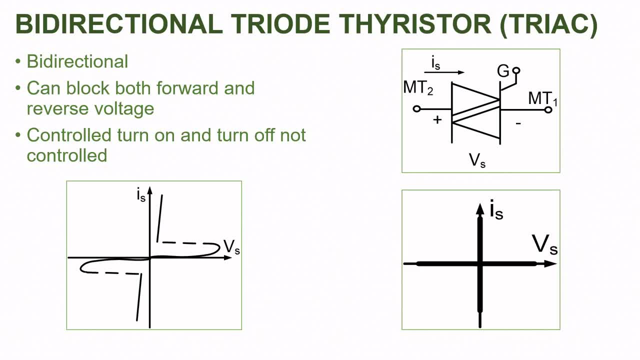 terminal MT2 is at a higher potential than MT1.. or when the terminal MT1 is at higher potential than MT2.. The turn on process of TRIAC can be controlled by giving signal to the gate terminal, but the turn off process of the TRIAC cannot be controlled by giving any signal to the gate terminal. 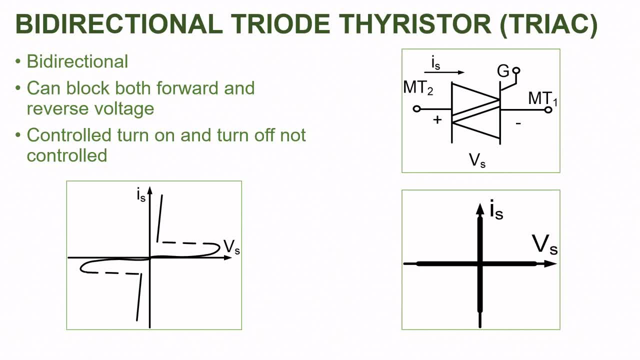 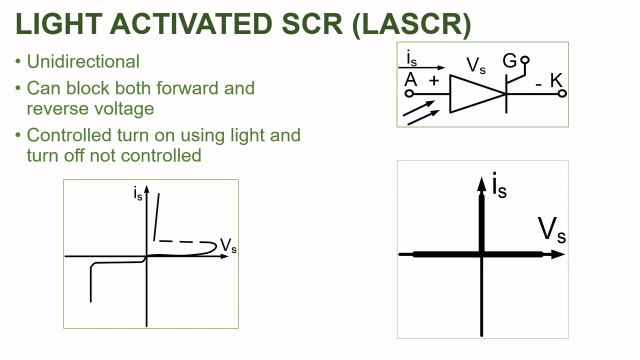 As you can see from the VI characteristics of triad, the VI characteristics of triad are identical in first as well as third quadrant. So our next device is light activated SCR, or LASCR As the name suggests. it is a type of SCR, hence similar to SCR. this device is also. 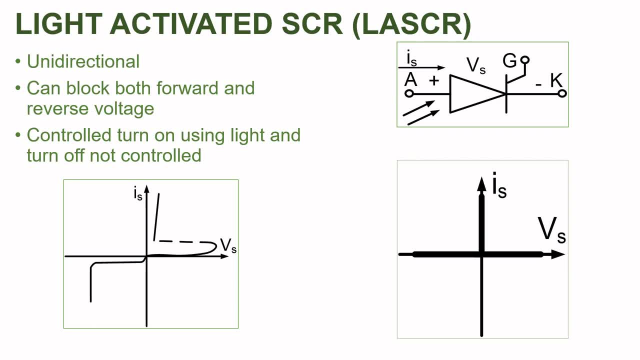 a unidirectional device. It can carry current only from anode to cathode and not from cathode to anode, But it can block voltages in both forward as well as reverse direction. The speciality of this device is turning on process. 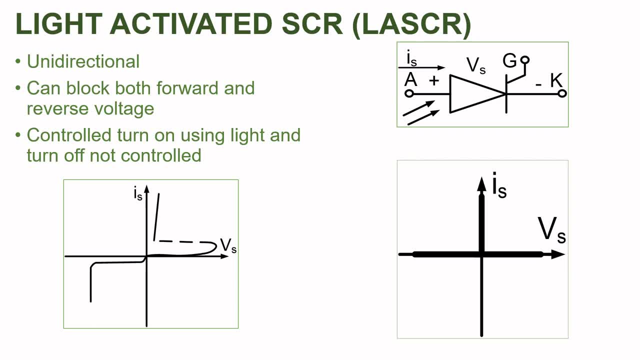 The turn on process of this device is not with the help of gate signal but with the help of light signals. In further videos we will be seeing the process of turn on of LASCR. The VI characteristics of LASCR are similar to that of VI characteristics of SCR. 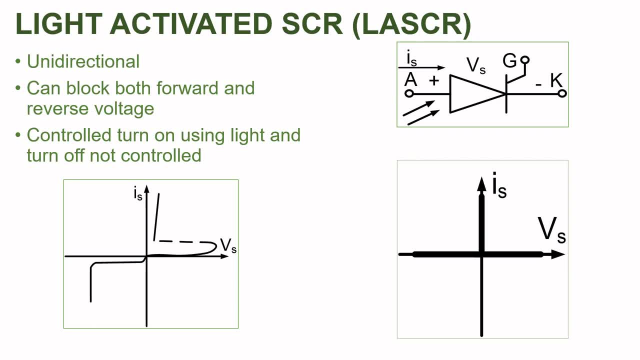 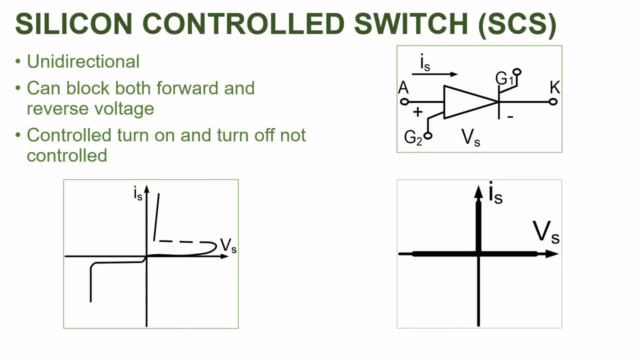 Silicon controlled switch or SCS. Silicon controlled switch is a unidirectional device. That means current will be flowing from anode to cathode and not from cathode to anode. Silicon controlled switch can block both forward as well as reverse voltages. 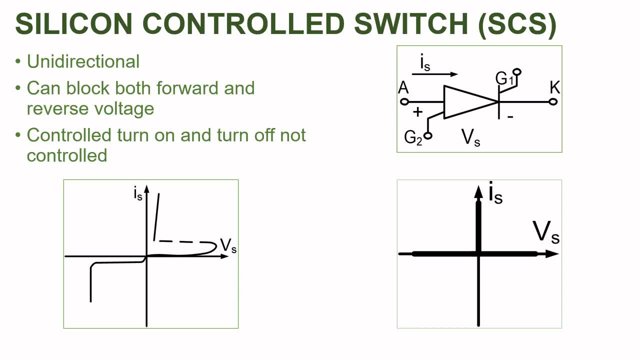 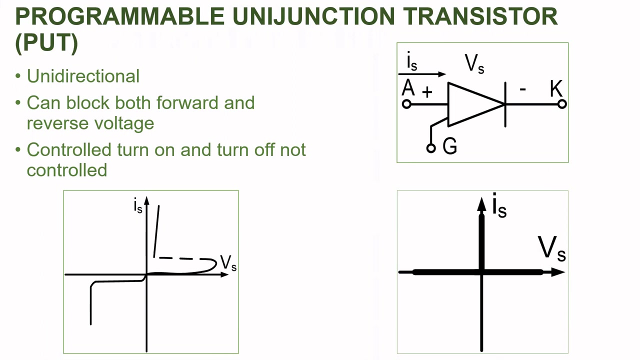 The turn on process of silicon controlled switch can be controlled by giving electrical signal to the gate terminal, But the turn off process is not controlled. VI characteristics of silicon controlled switch is somewhat similar to that of VI characteristics of SCR. Programmable Unijunction Transistor or PUT. PUT is a unidirectional device. It can block. 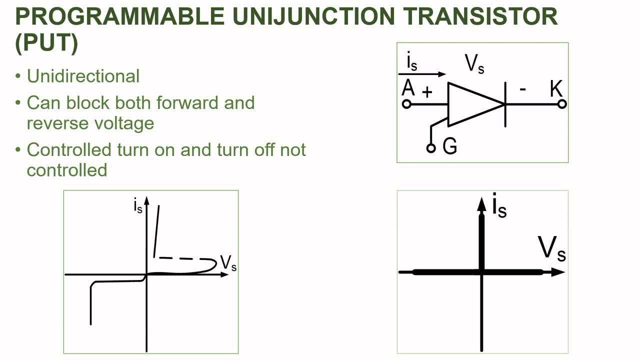 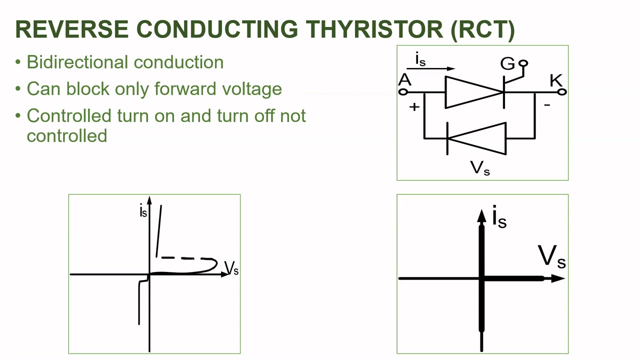 both forward and reverse voltage. The turn on process of the PUT can be controlled, but the turn off process is not controlled. The main application of PUT is in triggering circuits of SCR. Our next device is Reverse Conducting Thyristor, or RCT. RCT is a bidirectional device. That means it can conduct from anode to cathode. 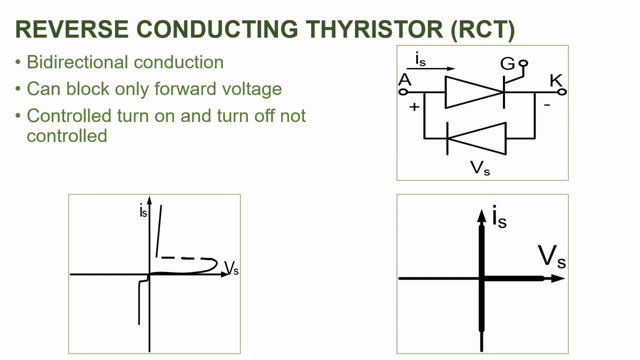 or cathode to anode, But RCT can block voltages only in the forward direction. That means when anode is at higher potential with respect to cathode. only under this condition RCT can block the voltage. As you can see from the symbol of RCT, there is a diode which is connected in anti-parallel combination with the SCR, So RCT can block voltage only in the forward direction. As you can see from the symbol of RCT, there is a diode which is connected in anti-parallel combination with the SCR, So RCT can block voltage only in the forward direction. 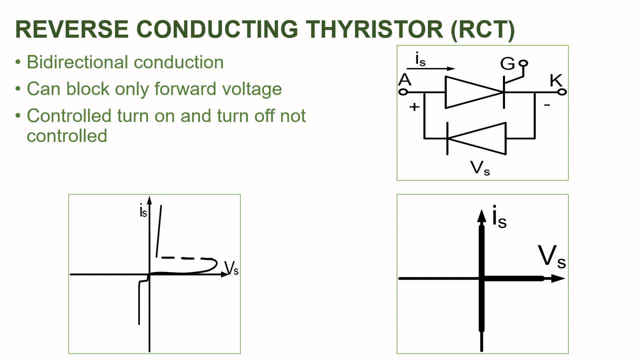 Whenever the device is forward biased in this condition, the SCR will then be able to block the forward voltage And since diode is reversed biased, the diode will not be conducting. But when the device is under the reversed bias condition we can say diode will start. 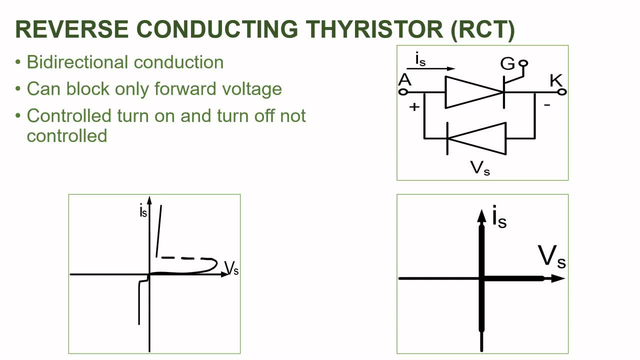 its conduction. When diode is reversed biased, side diodes fly in a eyelashes direction, The Barbara. The turn on process of the device can be controlled only under the forward biased condition. When the device is under reversed biased condition, the diode will be conducting immediately once. 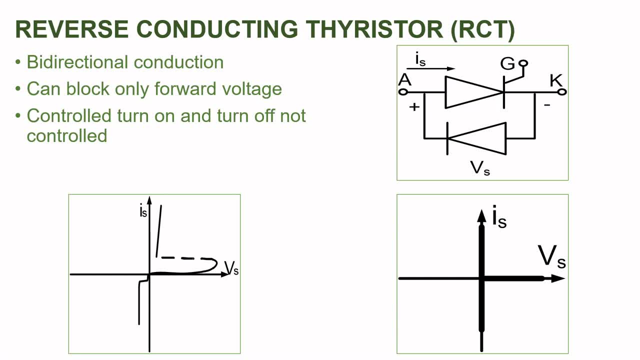 it gets forward biased, We will not be able to control the conduction of the device under the reversed biased condition. Turn off process of the device. though it is, turn off process of the device cannot be controlled in both forward biased condition or reversed biased condition. 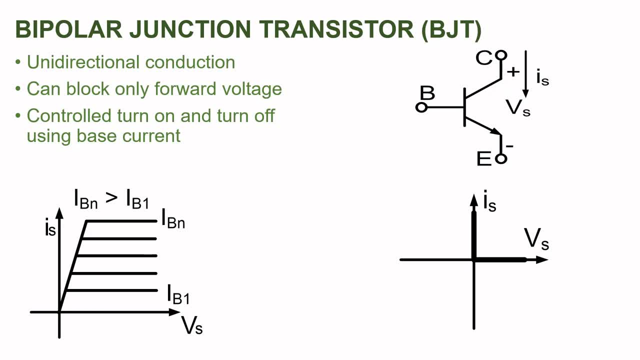 Bipolar junction transistor, or BJT. BJT supports only unidirectional conduction. that means current can be conducted from collector to collector. Also, BJT can block only forward voltages. that means when the collector is at higher potential with respect to the emitter, BJT can block the voltage. 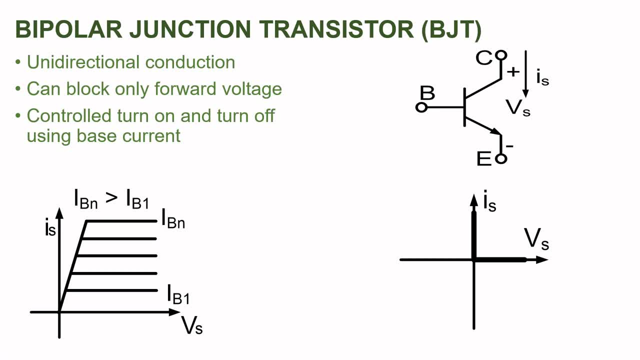 But the main advantage of BJT is: BJT is a fully controlled device. Both turn on and off process of the device can be controlled only under the reversed biased condition. The turn on process and turn off process of BJT can be controlled by using base current. 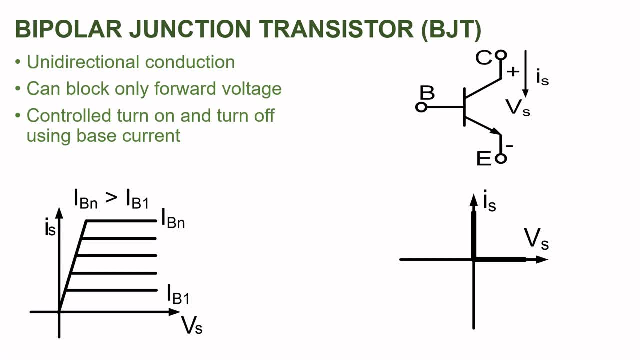 Whenever base current is given, BJT will start its conduction. Whenever the base current is removed, BJT will stop its conduction. The VI characteristics of BJT are as shown in the figure. These VI characteristics can be controlled by using base current. 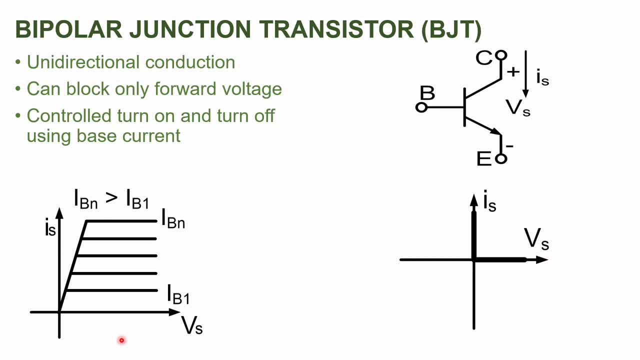 BJT 220G, 5G, 8G, 9G, 20G, 40G, 45G, 40G, 33G, 40G, 3G, 46G, 23G, 43G, 38 section, 396, 48弧. 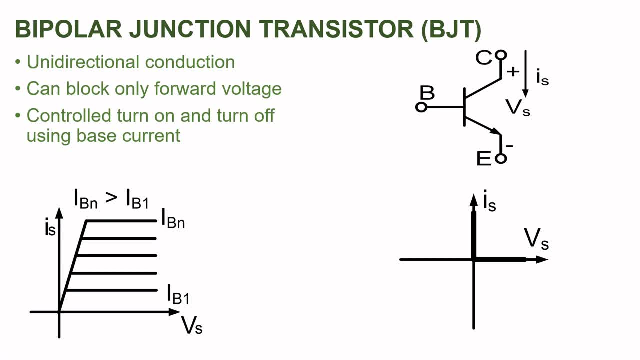 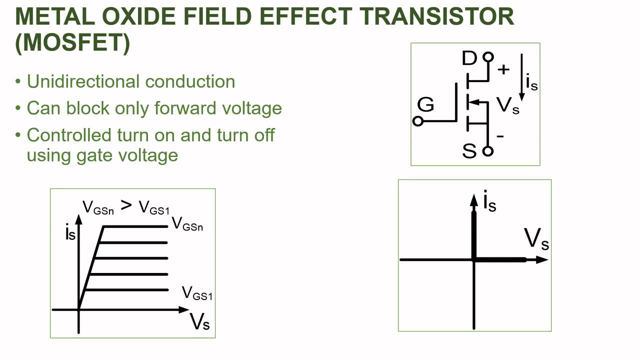 451, 30abulano, 33rap, 42, 351, 011, Prone, 32pt. utilized for the amplification purpose. Metal Oxide Field Effect Transistor, or MOSFET. MOSFET is a unidirectional device. It conducts. 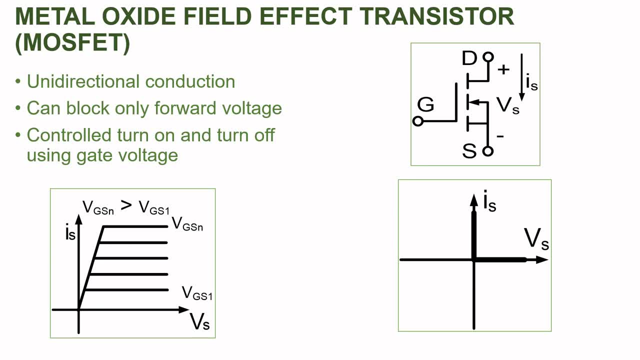 only in one particular direction. It can block only forward voltages. Advantage of MOSFET is it is a fully controlled device. That means both turn on process and turn off process of the MOSFET are controlled with the help of gate to source voltage. The VI characteristics. 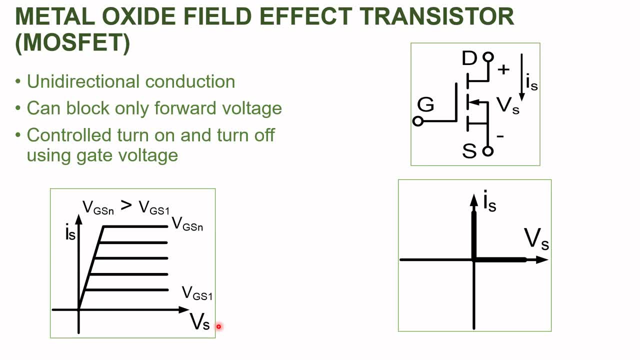 of MOSFET can be seen in the figure. These VI characteristics are similar to the VI characteristics of BJT, But the main difference is that the MOSFET is a fully controlled device. That means both turn on process and turn off process of the MOSFET are controlled with the help of gate-to-source. 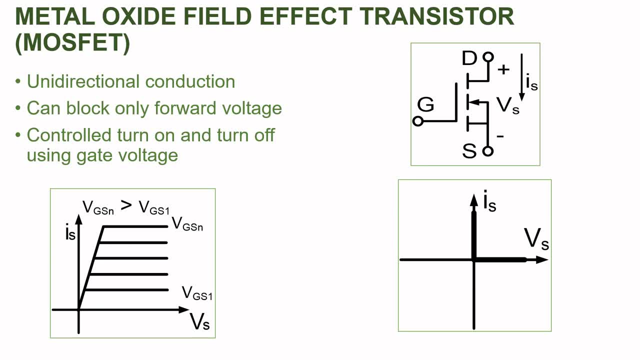 voltage. In case of MOSFET, the actuating signal is gate-to-source voltage and in case of BJT, the actuating signal is base current. Hence MOSFET is known as voltage control device and BJT is known as current control device. 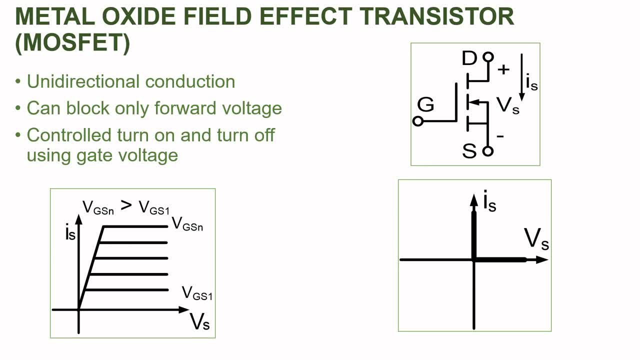 When we are going to use MOSFET in power electronic converters. we are going to utilize the MOSFET in the current control devices. So we are going to use the MOSFET in power electronic converters as a power electronic switch. So from the characteristics, we will be using only saturation region characteristics and 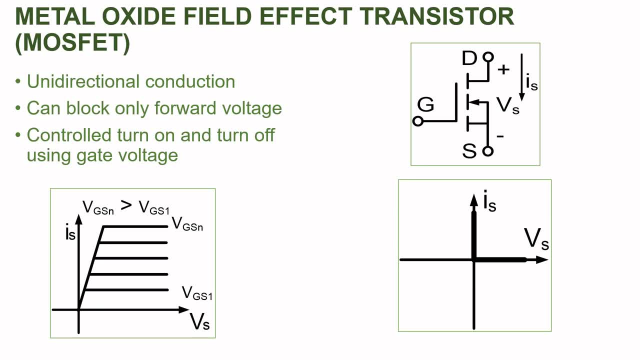 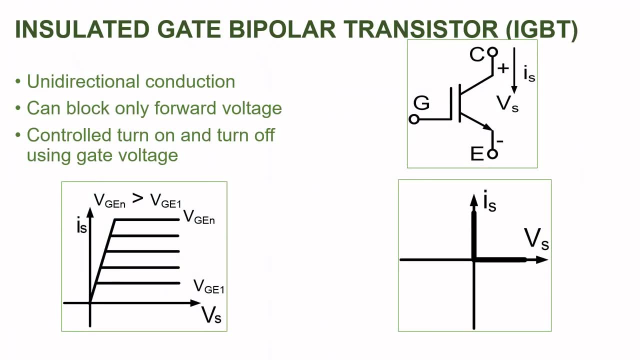 cut-off region characteristics. Active region characteristics. would not be used for power. electronic application Insulated Gauge Bipolar Transistor or IGBT. IGBT is IGBT-Cval nose. I hope it will be the most common type of MOSFET. We are not. going to use it for any power electronic application. We are going to use it for made of transformer. ating length of time. So the type and diameter of IGBT is IGBT. IGBT is IGBT-Cval nose. IGBT is IGBT-Cval nose. 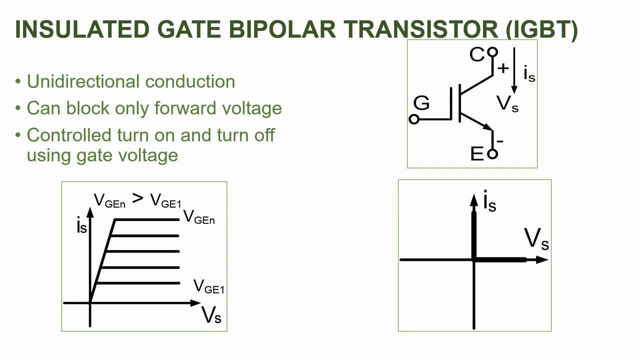 IGBT allows only unidirectional conduction. IGBT can block voltages only under the forward biased condition. Similar to BJT and MOSFET, IGBT is also a fully controlled device. that means both turn on and turn off process of the IGBT can be controlled with the help of gate to emitter. 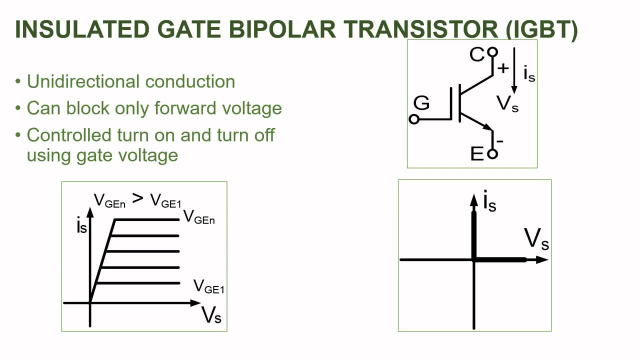 voltage VI. characteristics of IGBT are shown in the figure. Similar to MOSFET, IGBT is also a voltage controlled device. When we are going to use IGBT And in the power electronic converter we are going to utilized saturation region and cut. 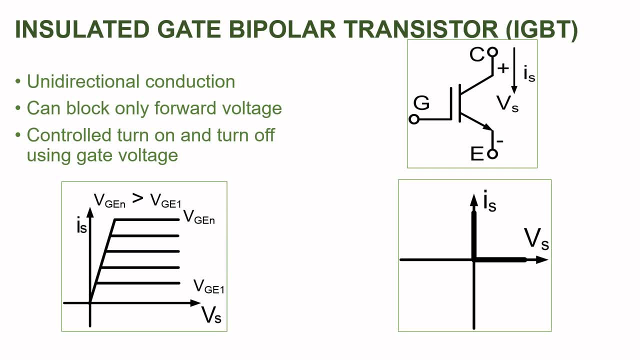 off region of the characteristics. Active region of the characteristics would not be used in power electronics. IGBT has the advantages of both MOSFET as well as BJT. I was doing an experiment. What is it? Yes, Yes, No. 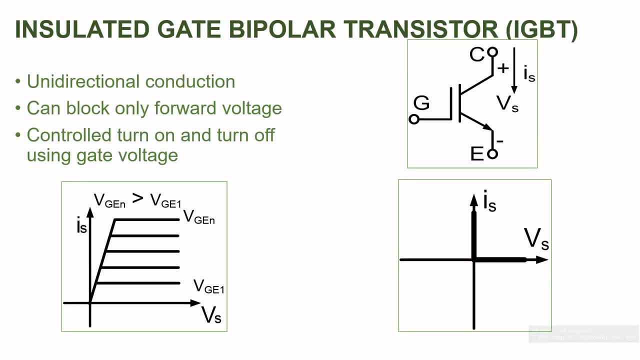 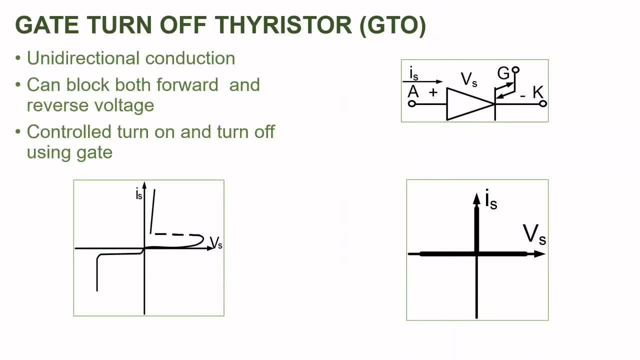 No, No Gate Turn Off Thyristor or GTO. GTO is the device which allows conduction only in one direction, that is, from anode to cathode. GTO can block voltages in both forward as well as reversed condition, Unlike other devices from the thyristor family, which can be turned on with the help of gate. 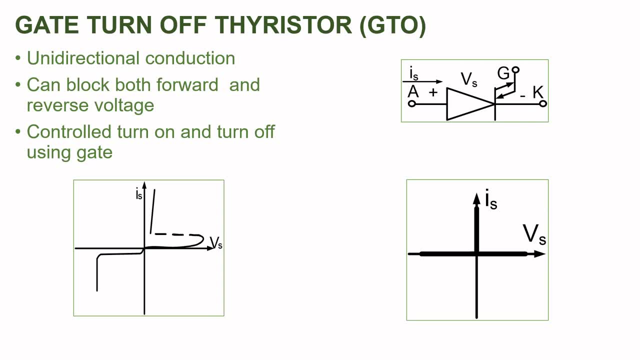 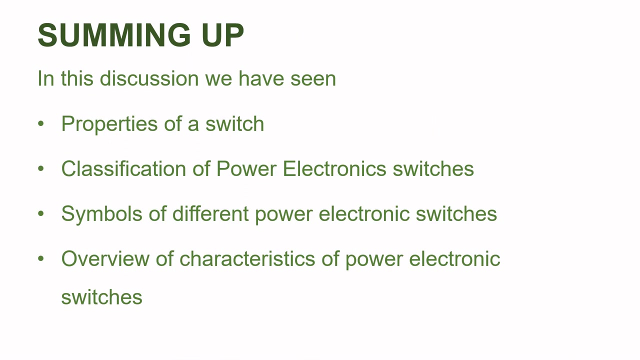 and after turning on gate loses control over the operation of the device. In case of GTO, both turn on process and turn off process can be controlled by using gate signal. In this discussion we have seen properties of a switch, classification of power, electronic. 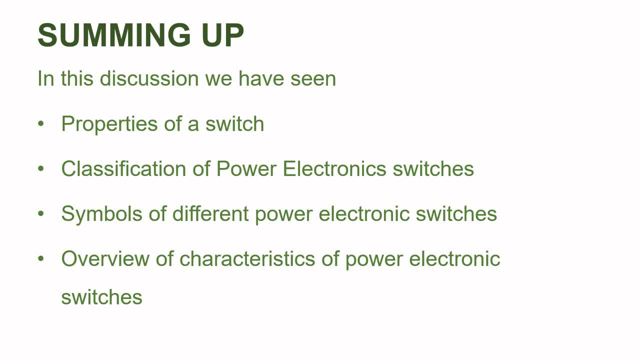 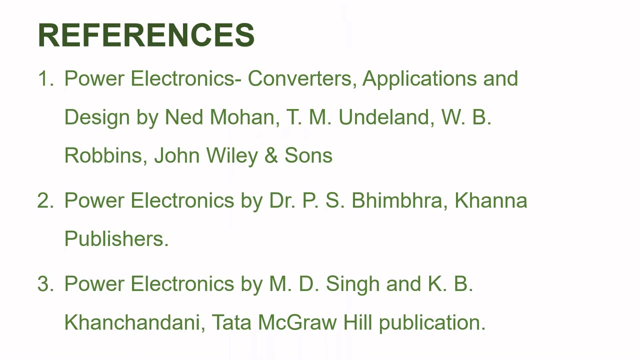 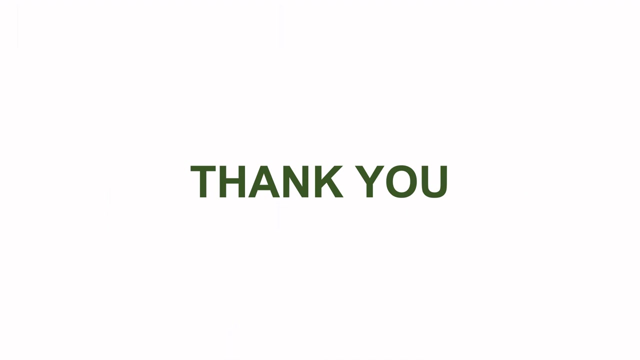 switches. symbols of different power. electronic switches. Overview of These are some references which we have used for creating this presentation. Thank you. If you like this video, please do hit the like button, subscribe button and share this video. Also, don't forget to press the bell icon so that you will be keep on getting the notification. 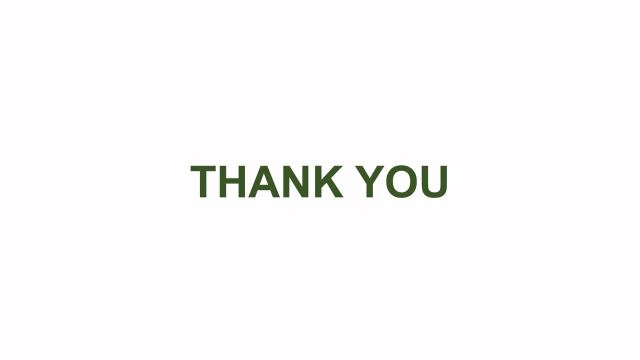 whenever we upload the new video. Thank you.